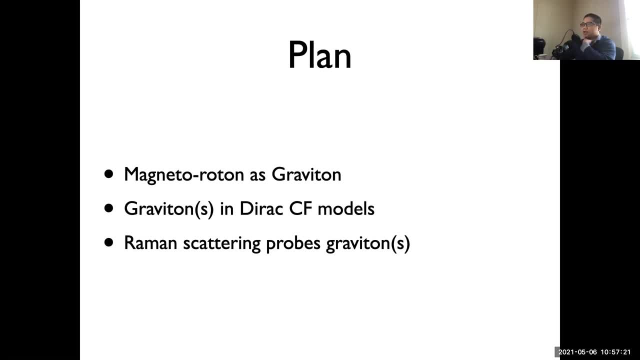 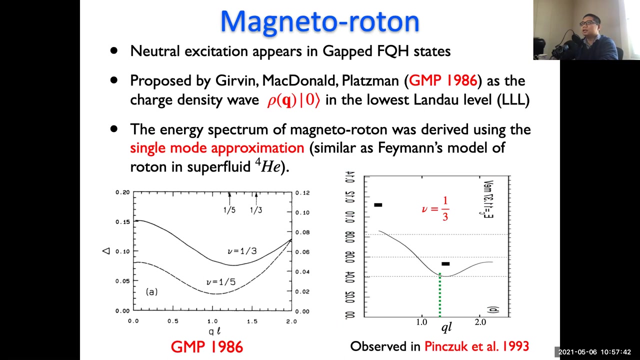 And then I will discuss that in the Dirac composition model maybe there are more than one gravitone mode, And in the last part of my talk I will discuss how to probe the gravitone mode using Raman scattering. So basically, you see that. 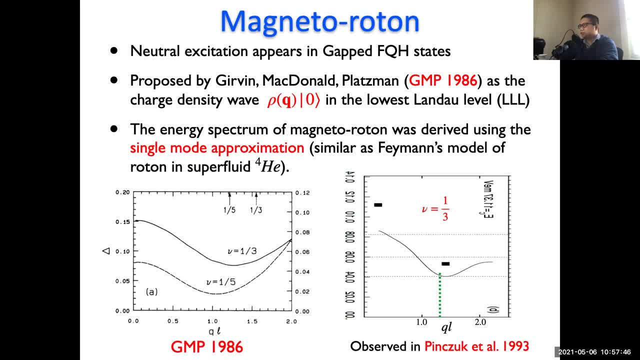 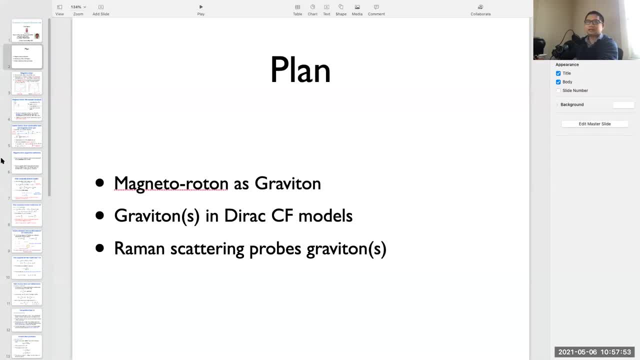 By the way, I think we cannot see your pointer. I thought I told you we can see it, but now we can't see it. So maybe, if you can share and share, I think maybe the same issue I had, share the full. 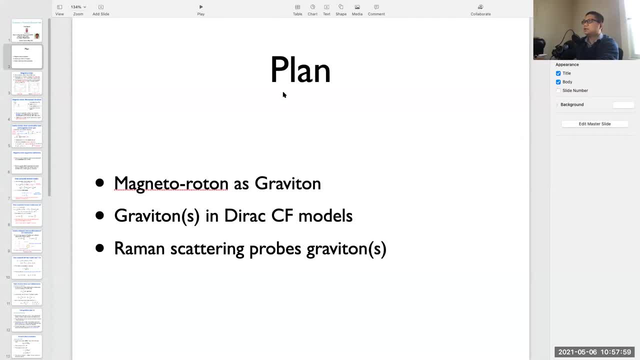 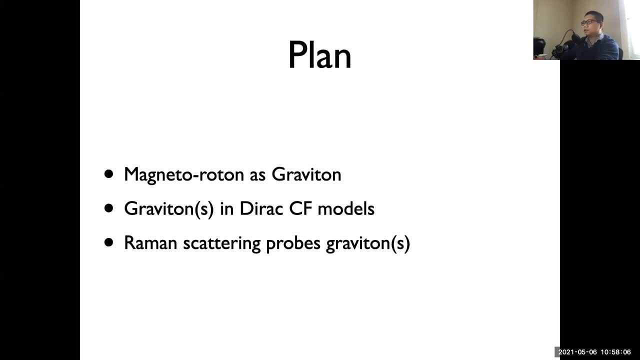 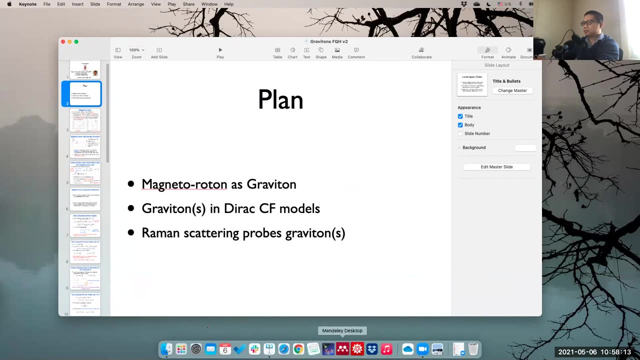 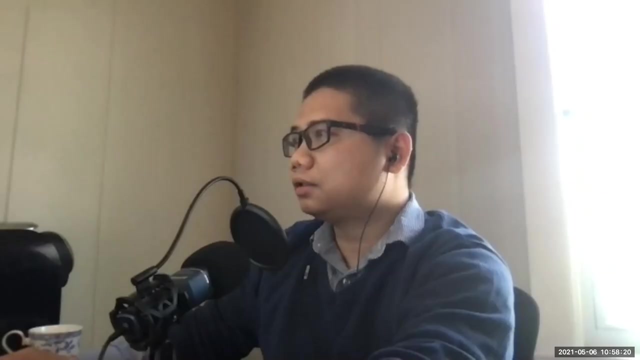 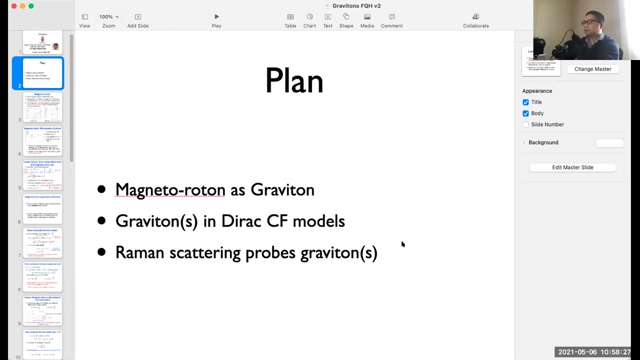 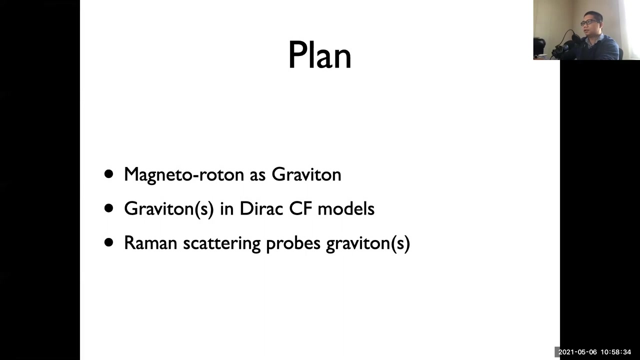 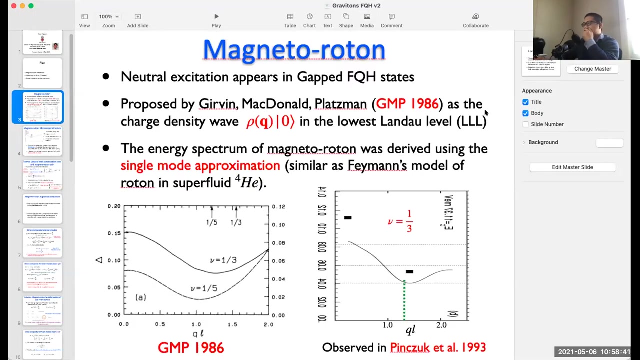 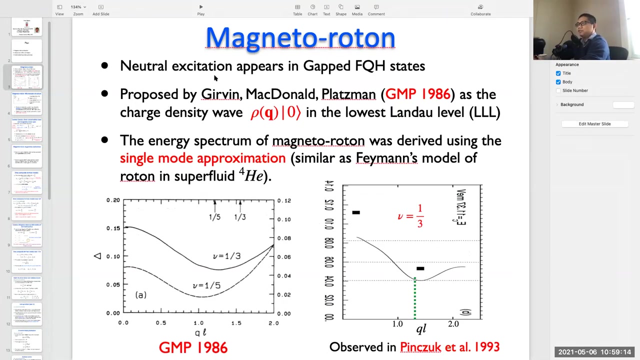 Okay, Okay, Can you see my pointer now? Yes, Disappeared right now, But can you move it in? Okay, Disappear somehow. I think you mentioned that if you share the, We know that In in the fashion of quantum Hall, we have the neutral excitation, which is a magnetrotone. 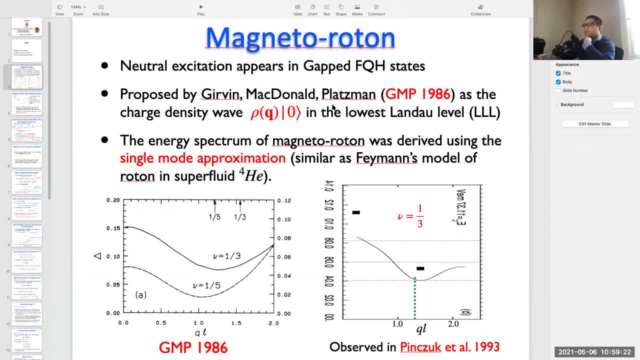 And it's were proposed by Govind, Macdonald and Plasman in 1986 as a charge density way. When you act on the ground state by the density operator, you increase the magnetrotone And the energy spectrum of magnetrotone was derived using the single most approximation, in the same manner as Feynman derived his roton in fluid helium-4.. 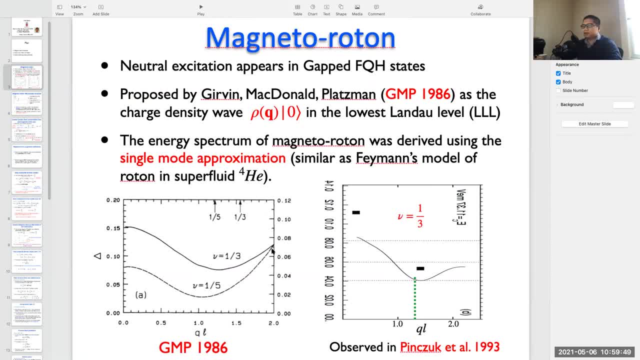 So here is a dispersion of the magnetrotone calculated by Govind, Macdonald and Plasman, And the magnetrotone dispersion after that was confirmed experimentally by group of Pinchuk In 1993.. So here you see the dispersion duration. 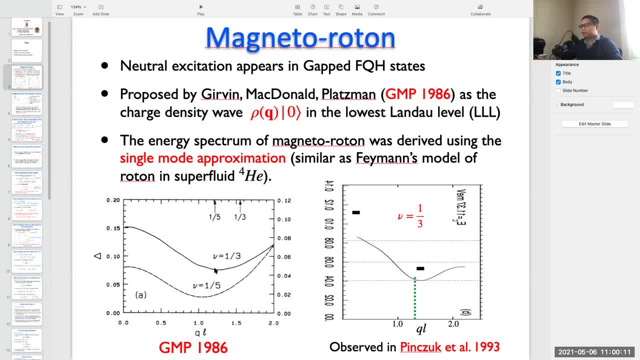 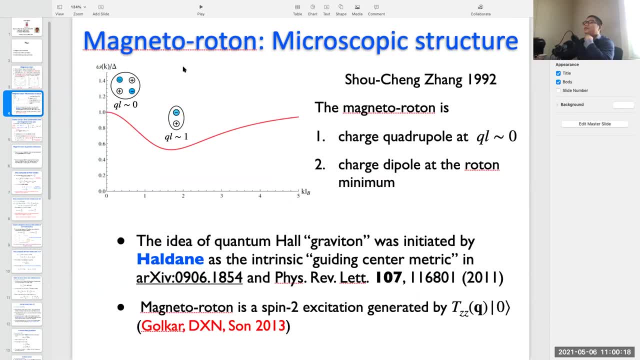 Let's look close to the theoretical proposal And further than that. the magnetrotone also have like microscopic structure And in the paper in 1992, Professor Chen Zhang suggests that the magnetrotone, when momentum close to zero, is a quadrupole. 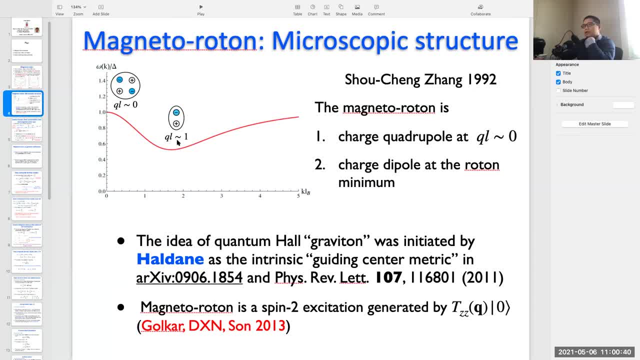 And when the momentum close to 1 over Lb, you will have the dipole near the minimum of the dispersion. And basically the idea of quantum Hall graviton was initiated by Houghton as an intrinsic writing sensor matrix In this paper in 2009, and also in the PIR paper in 2011.. 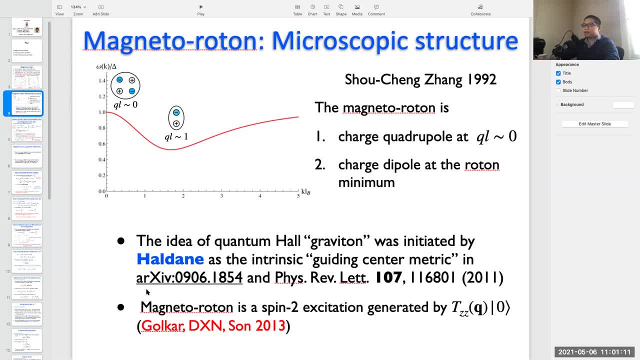 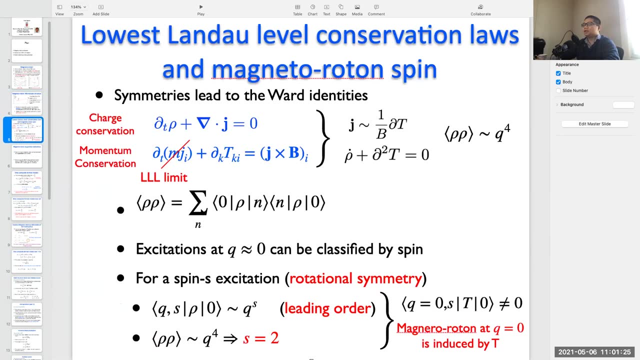 And we follow the idea by Houghton And in this paper with Gorkha and Cern, we suggest that the magnetrotone is a spin-2 excitation generated by the stress tensor operator axon-Grawstedt. And now I will explain why we think that is true. 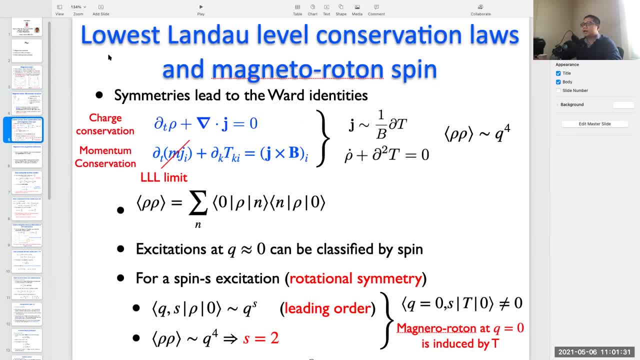 So here I show you the lowest Landau level conservation law. So the first equation is familiar with everybody, It's just nothing but the charge: conservation. So rho is the density and j is the current, And the second equation is the momentum: conservation. 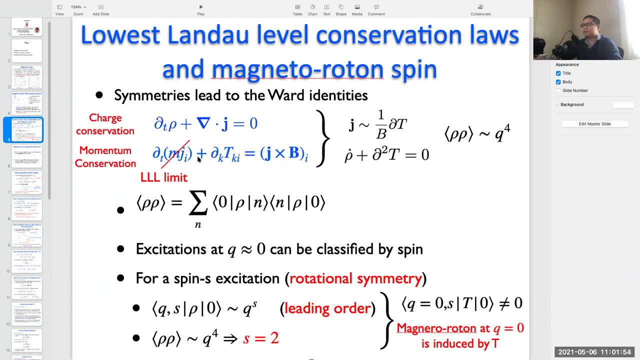 Where here m, multiplied by j, is the momentum And we have the derivative of stress tensor in the right hand side. In the right hand side is the Lorentz force. However, a mathematical way to go to the lowest Landau level is taking the electron mass. go to zero limit. 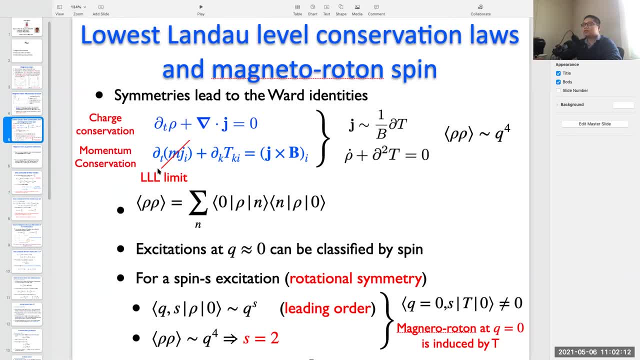 And in this situation we can ignore the first term And with the force balance term we can calculate the current in terms of the derivative of stress tensor in this way. So from that you see, that's the variation of density related to the force balance term. 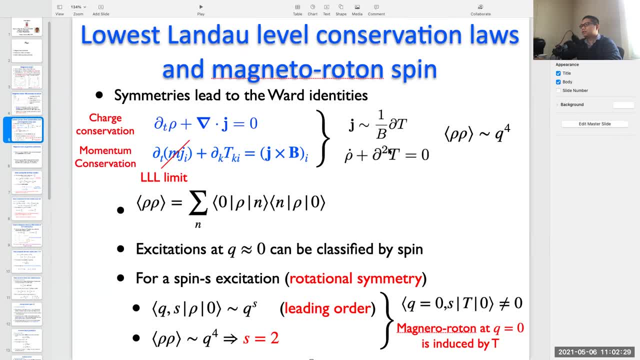 So we can use the derivative twice of the stress tensor in space. So that's why in this case we see that the density density correlation function should go as the Q to the force, If the stress tensor correlation function doesn't have any singularity at Q to zero. 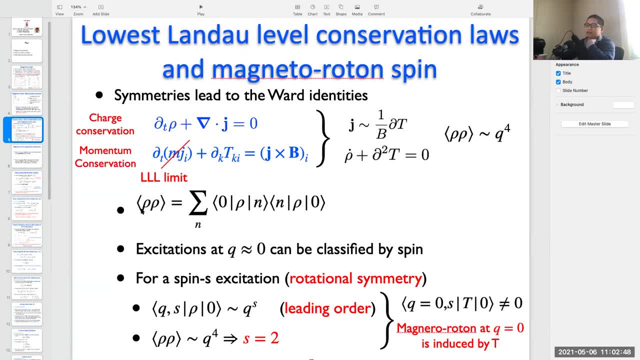 Okay, And we also can realize the correlation function here in terms of, like some, of the spectrum. And so basically from that we see that the excitation when momentum close to zero can be classified by spin. So for spin S excitation, you see that. 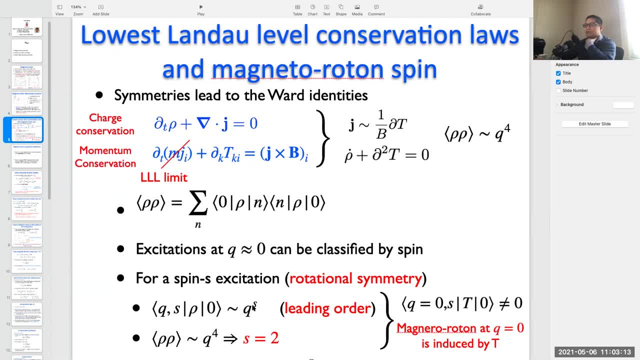 this magic element go as Q to the S. when Q goes to zero, The reason is because of the rotational symmetry. So rho is a scalar, So you need to contract the scalar from the spin and momentum. When you are contracting the index, you see that this magic element will go with the Q to the S if excitation has spin S. 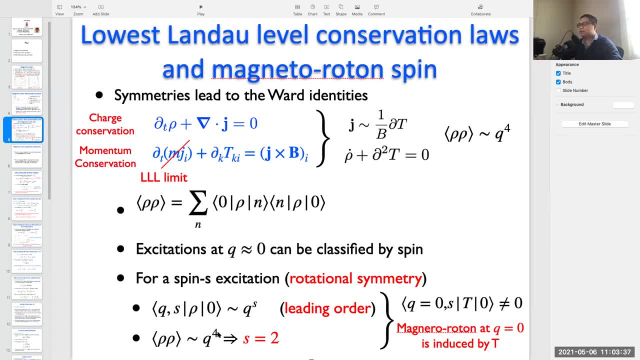 And so, because of the rho-rho correlation function calculated in the Wilman-McDonough paper, you see that it goes to Q, to the fourth. So that's why the spin of excitation is equal to two. Okay, And from this equation, 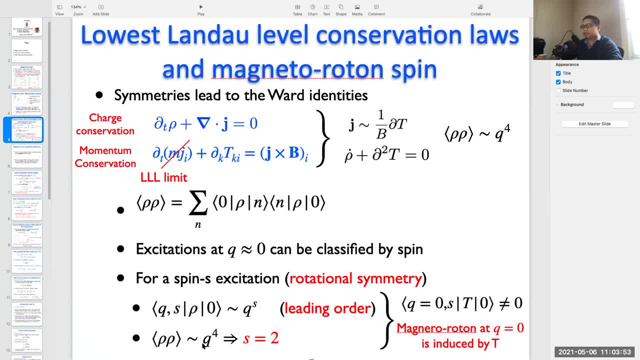 we see that with rho-rho go to Q, to the fourth, then that means this magic element is non-zero when Q goes to zero. Okay, And so basically we argue that the magnetroton at Q goes to zero is induced by the stress tensor operator. 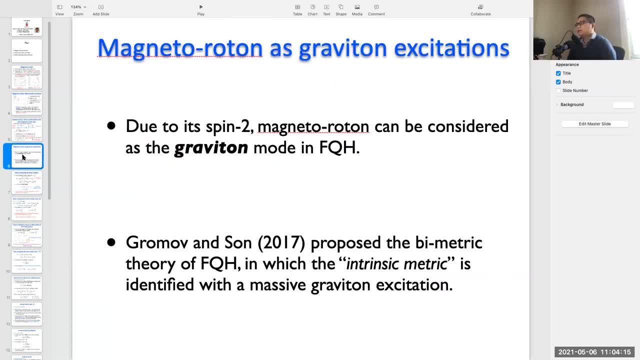 And, due to its spin tool, magnetroton can be considered as the graviton mode in the fractional quantum Hall And actually in the paper in 2017, Andre and Son proposed the biometric theory of fractional quantum Hall effect, in which the intrinsic metric is identified with the massive graviton excitation. 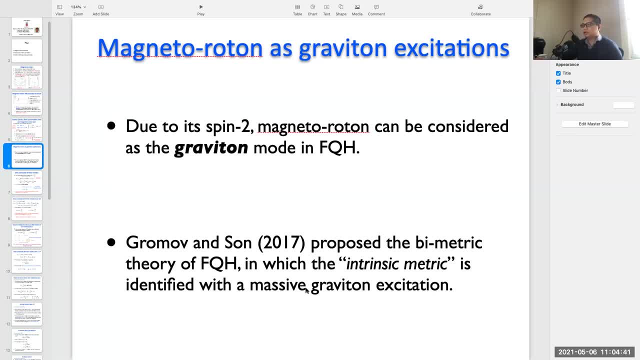 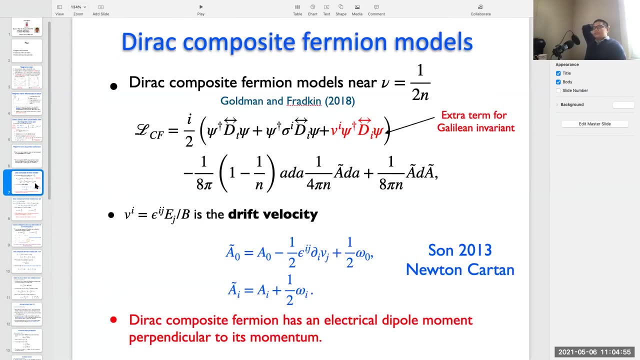 And in the subsequent paper we saw that the intrinsic metric is also corresponding to the magnetroton mode. This is the gravitational quantum Hall effect. Okay, so the main part of this talk. I will discuss the spin tool modes in the composite fragment module with the filling fraction near 1 over 2.. 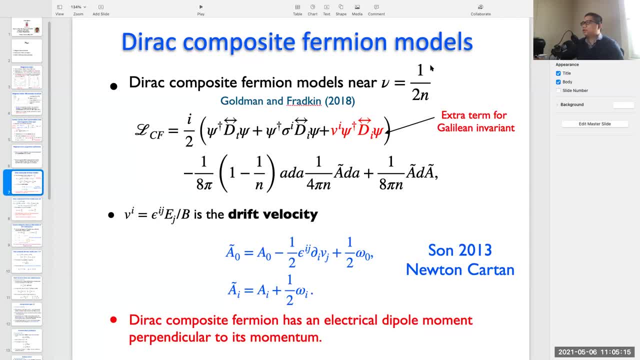 So we discuss the graviton mode of the JN sequence, the general JN sequence. Okay, Okay, Thank you. Thank you very much, Thank you very much. Okay, So we have the composite-familial model introduced by Goldman and Fratkin, with this form: 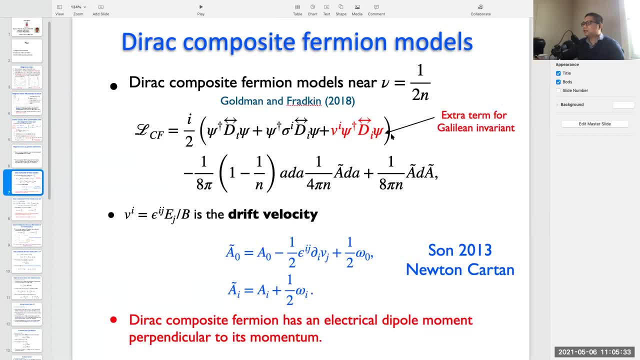 And here I just add an extra term for the Valiant invariant, which Vi is nothing but the drift velocity calculated in terms of electric field and background magnetic field. So from this term you see that the Dirac composite-familial has a dipole moment. 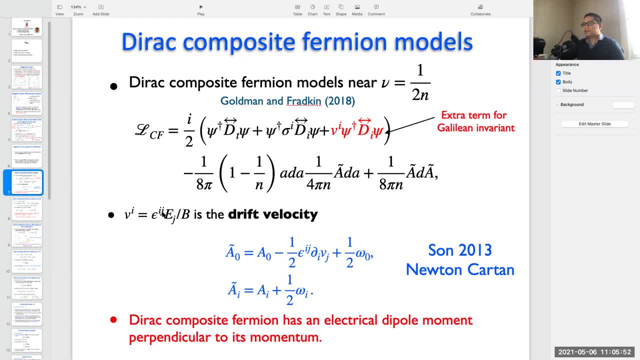 And because of this, this epsilon coefficient, epsilon ij, here we see that the dipole moment of the composite-familial perpendicular to its momentum, And here we have the improved A tilde defined in certain Newton-Cartan formalism. So from this model, now with n, with the coefficient small n here, if we go to n equal. 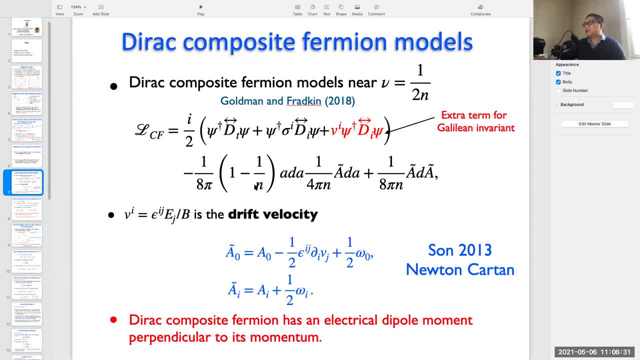 to 1, small n equal to 1, that means we study the Dirac composite-familial model near half-filling. In this case we don't have the IDI term and we put n here equal to 1.. 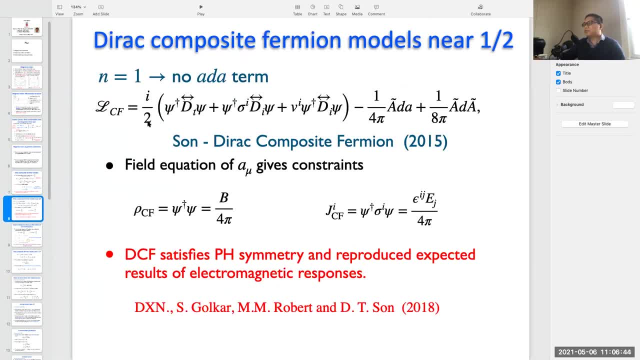 And here is the Lagrangian for the Dirac composite-familial model. And here is the Dirac composite-familial model. The Dirac composite-familial model is nothing but the Dirac composite-familial model. And from this equation, from this Lagrangian, you see that both composite-familial and the 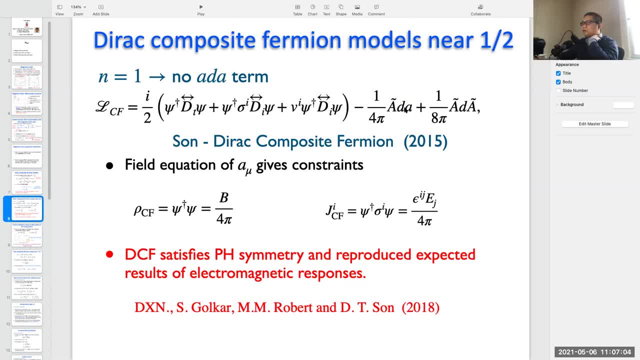 external field couple linearly with the small a, with the emergent gauge field. So the field equation of emergent gauge field gives us a constraint. So from this we see that when you variation this Lagrangian with respect to small a naught, you see that the composite fermion density equal to the magnetic field divided by four pi. 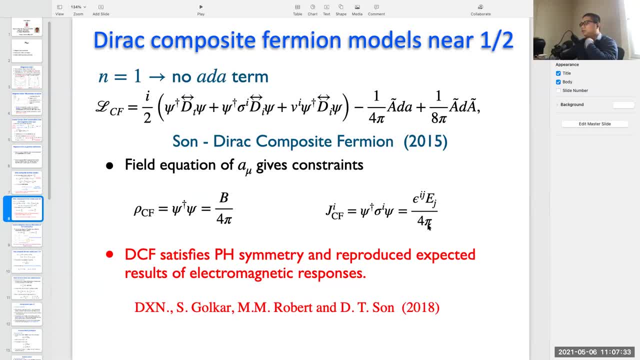 And furthermore the composite fermion current related to the applied electric field And from this model we saw in my other work with Gorka, Robert and Son. we saw that this Dirac composite fermion model satisfies the particle-hole symmetry and also reproduces the expected result of electromagnetic response. 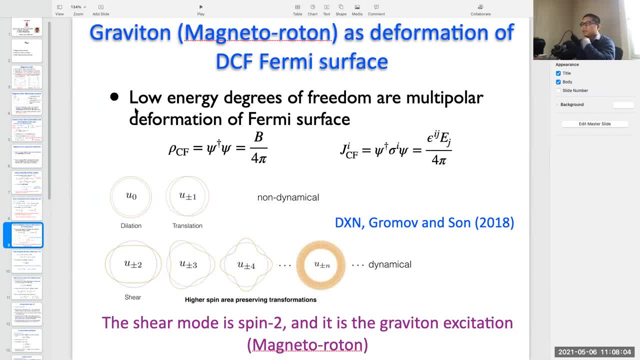 And now we see that the low energy freedom of this Dirac composite fermion model, as a multipolar deformation of the fermion surface, of the composite fermion surface- And here is a figure that I borrow from Andre in many of his talk- and because of the Dirac composite fermion density is fixed by the applied magnetic field and the composite fermion current fixed by the applied electric field. 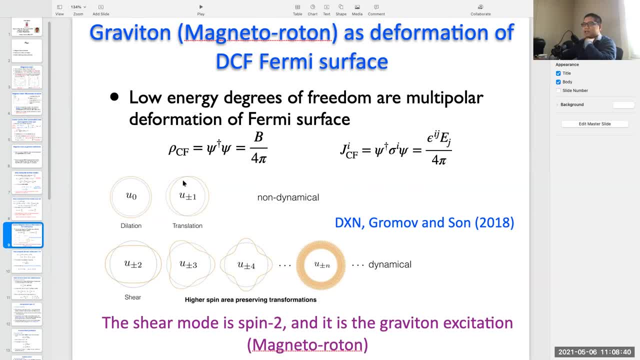 So That's why the dilatation mode and the translation mode of the deformation of Fermi surface is non-dynamical, because it's constrained. However, you can have all other higher deformation of the direct composite Fermi surface And basically, in my paper with Andre and Son in 2018,. 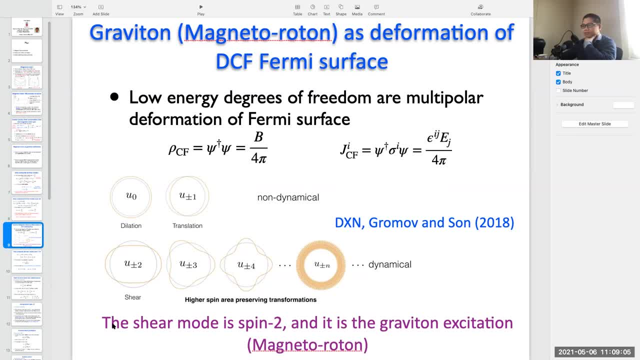 we saw that the biometric theory mode correspond to the shear deformation, and with a spin too, And so we identify that the immersion, the immersion degree of freedom at low energy, here has a spin too, and it's a magnetroton and it's nothing. 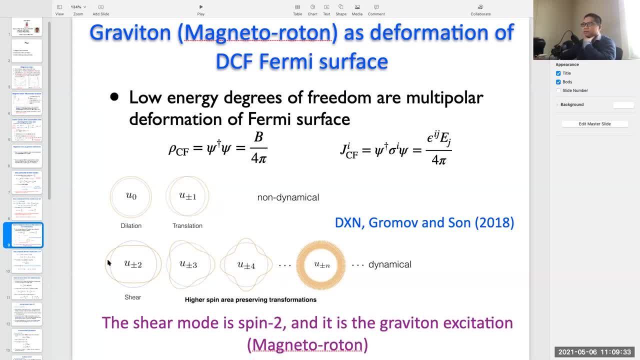 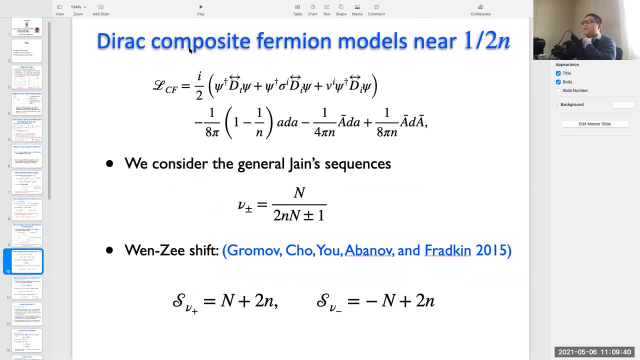 but it's a deformation of direct composite Fermi surface, the shear mode. So now we come back to the model with the average small N, For example one-fourth, one-sixth or one-eighth, and caterpillar, And we consider the two-gain sequence. 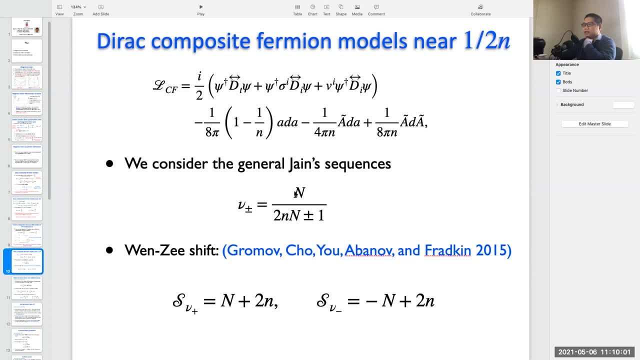 with this filling fraction where N do it to infinity, 8P and 3P- And with this fling fraction of the chain sequence, we already know the Wenzhi shape, calculated in this paper by Andrei Chou, Yu Sasha and Eduard Fratkin. 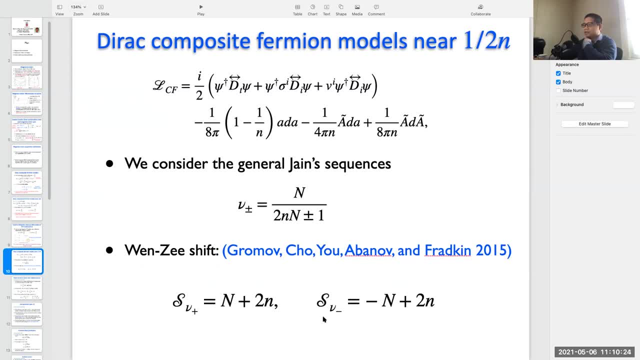 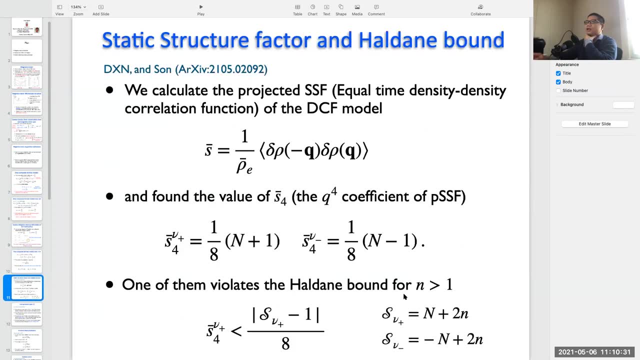 Here is the equation that determines the Wenzhi shape. Okay, And from this Dirac-Composite framework model, introduced by Goldman and Fratkin, we can calculate the projected static structure factor, which is nothing but equal time density-density correlation. And we see that with this definition, you will get the value of the coefficient. 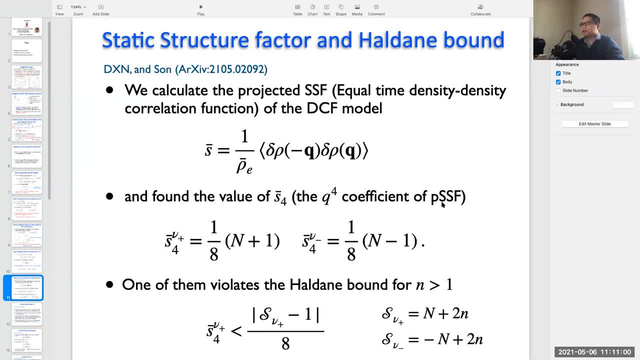 S4 is the coefficient of Q to the fourth in the projection. So we can calculate the projected static structure factor with this form. Okay, And there's one issue that happened here. So Hauden in some paper suggests Hauden-Bow for the S4 of the static structure factor. 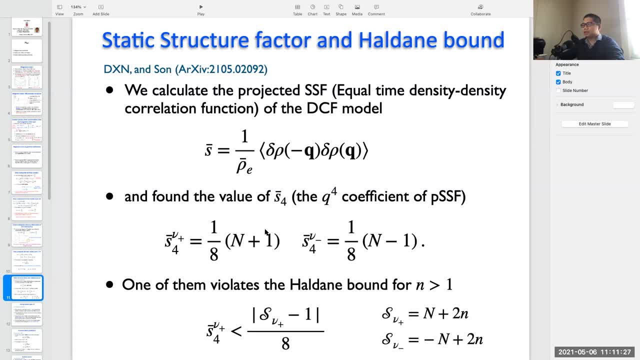 And we see that with this result of the static structure factor, the Dirac-Composite framework model, we see that it violates the Hauden-Bow for the fling fraction nu plus here. Okay, So with n bigger than 1, then you see that you violate this because the result here is smaller than the right-hand side. 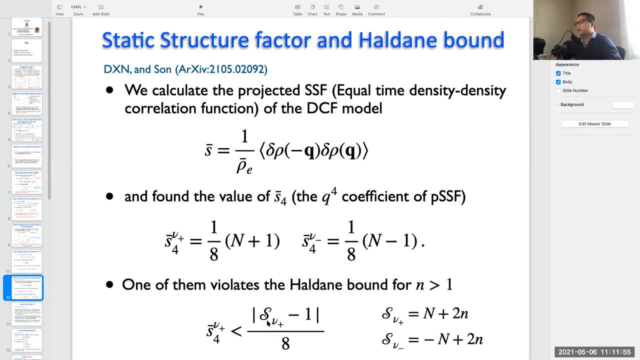 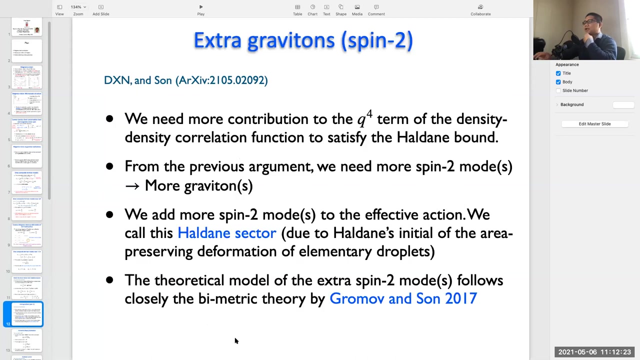 It's not the problem of the Dirac-Composite framework model, near half-filling with small n equal to 1. Because at this time this sign will be the equal sign. So it's not the problem. And now, motivated by the argument on the density-density correlation function and the spin of the excitation, 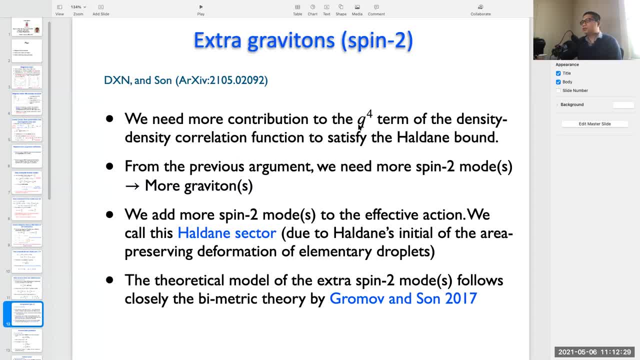 we see that we need more contributions. Okay, So from the previous argument about the spin of the excitation, then we need more spin-to-mode, so we need to have more graviton. Okay, So to do that, we add more spin-to-mode to the effective action. 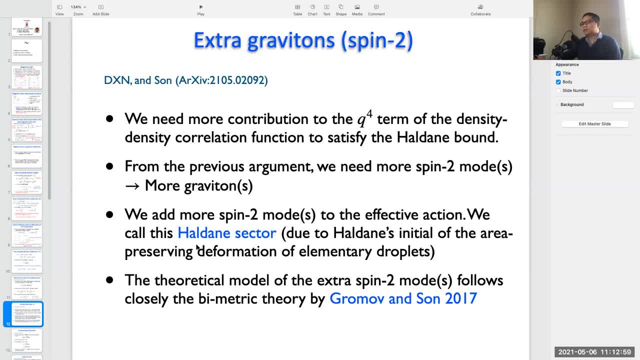 And we call the extra spin-to-mode. The extra spin-to-mode is the Hauden sector due to the Hauden initial idea of area-preserving deformation of the elementary droplets. However, the theoretical model of the extra spin-to-mode follows closely the biometric theory by Andre and Cern. 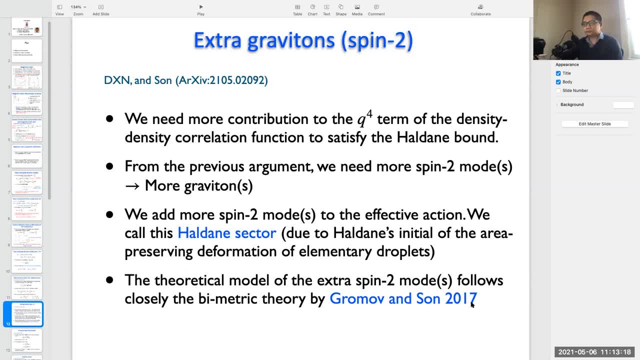 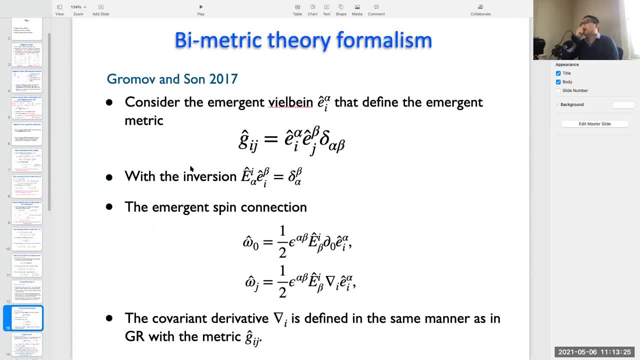 Okay, And in the biometric theory, formalism, we consider the extra degree of freedom with this immersion view-by And from that the view-by also can be defined through the new immersion matrix. Yeah, So this is the idea introduced by Andre. 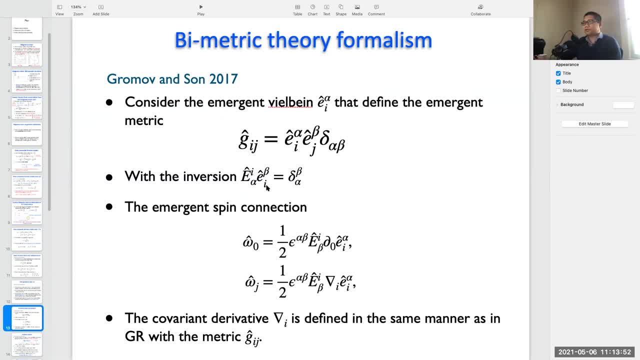 And from that we also have the inversion view-by And define the spin connection, the immersion spin connection, in the usual way Here this is nothing, but it's the covariant derivative defined in the same manner in the GR with the matrix GH IJ. 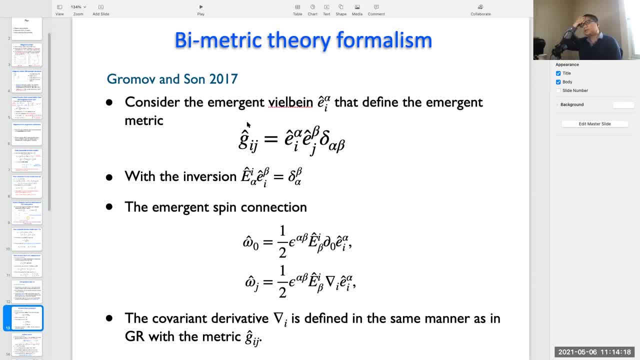 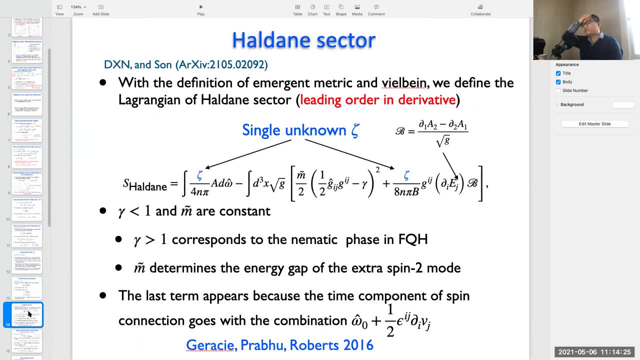 It's nothing, but it's the immersion matrix. Okay, So here is our proposal for the Lagrangian of the Hauden sector. So the Lagrangian of the Hauden sector have this form. So A is the background magnetic field. 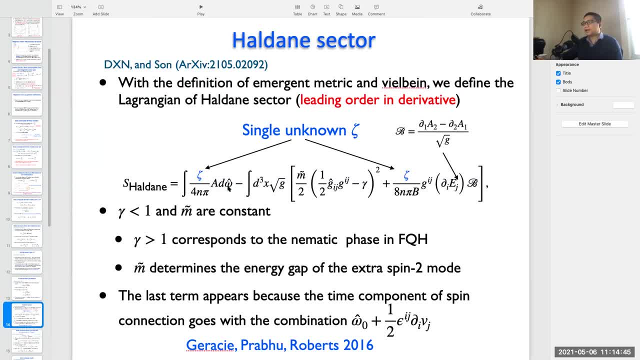 The background, base field And omega hat. here is nothing, but it's the immersion spin connection that we defined in the previous slide. Okay, And finally, we have the Lagrangian of the Hauden Thecast vantage, the. So the Lagrangian. this Lagrangian is nothing but is leading order in the derivative of the Lagrangian of bimetric theory that's introduced by Andre and Eun-Seo Son in 2017.. 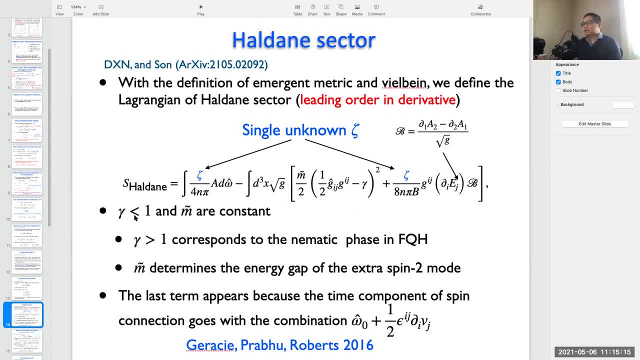 Okay, So here we have a few constant. Are we gay? we are in the isotropic phase of the fractional quantum hole, and m tilde is also positive and constant. However, the important coefficient here is the single unknown zeta And basically the last term here. 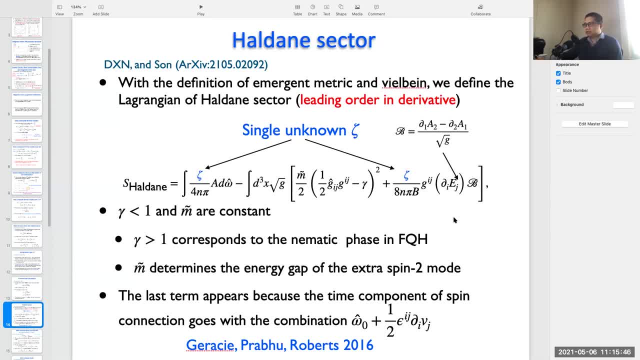 will appear because of the time component of the spin connection will go with the combination with the extra term. here is the vorticity of the deep velocity here And basically we need to emphasize that there's only a single unknown in this Lagrangian. 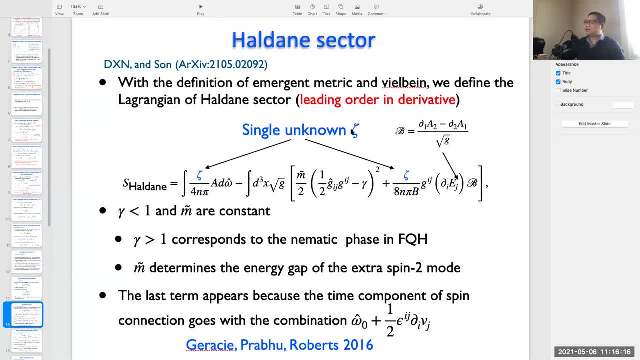 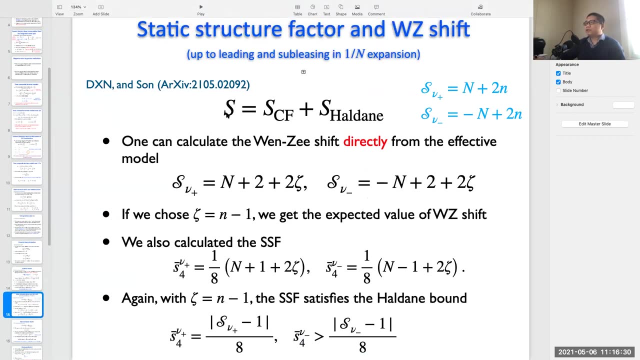 And we need to find the single unknown here that is only depend on small n. And now, with the full theory, including the composite fermion sector introduced by Goldman and Fratkin, we add the Horten sector here and we can create the Wenzhen. 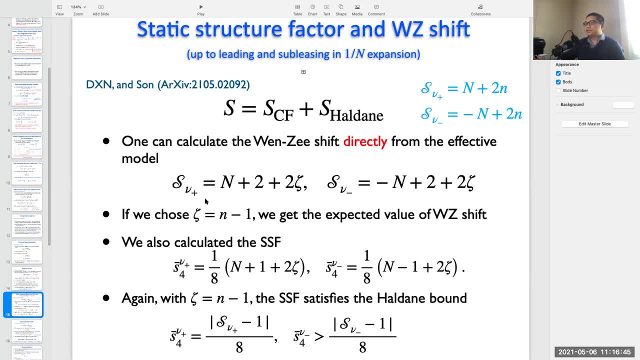 shift directly from the Horten sector And we can create the Wenzhen shift directly from the Horten sector here. and we can create the Wenzhen shift directly from the Horten sector And we can create the Wenzhen shift directly from the Horten sector And we see that the Wenzhen 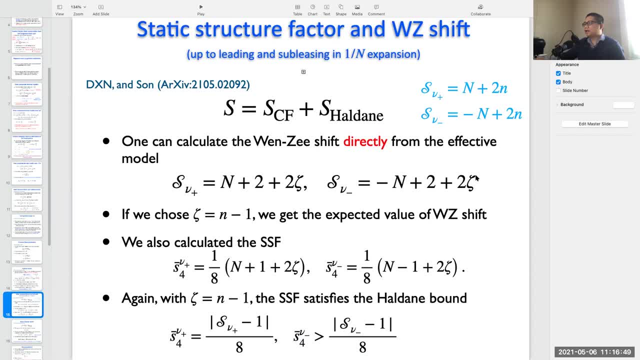 shift has this form, with the eta for both mu plus and mu minus. Now we compare with the known result for the Wenzhen shift of the jane sequence. We see that if zeta equal to n minus one you get the expected value of the Wenzhen shift And you see that near half failing. 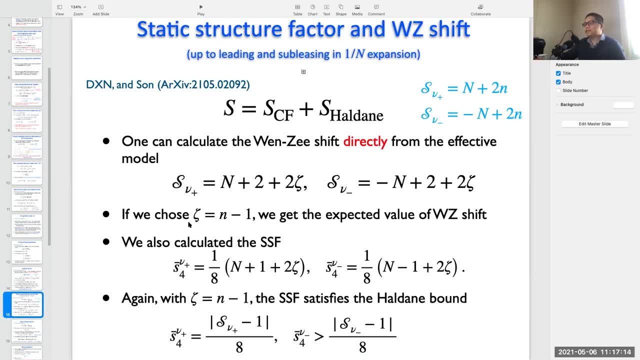 when n equal to one, you see that zeta equal to zero and that means we don't need to to consider the Horten sector. And from the full theory we also can create the static structure factor and it is a form of the static structure factor. 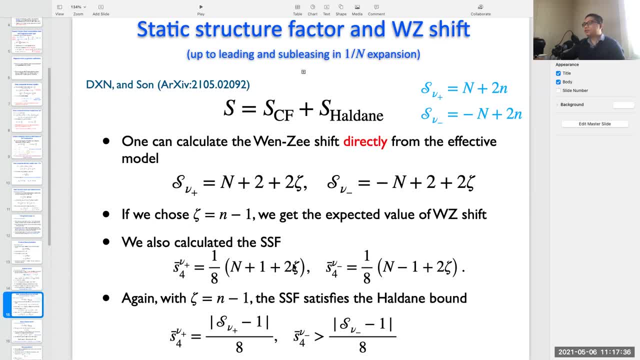 including the new term zeta. It's a contribution of the Horten sector to the static structure factor calculation. And again, if we choose zeta equal to n minus one, the static structure factor satisfies the Horten bar. So the new plus, we saturate the bar, but the new minus higher than the bar. but it's also okay. 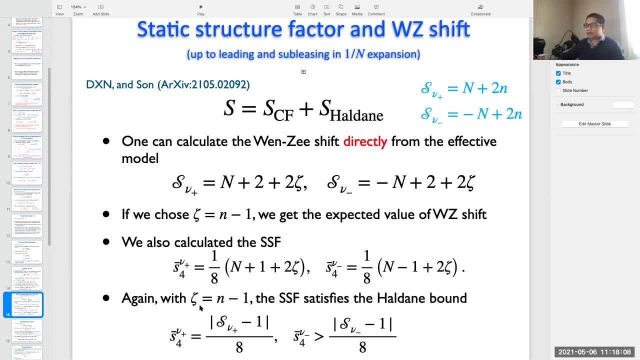 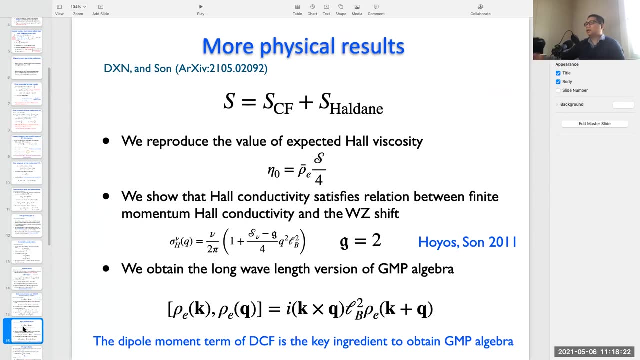 So in the previous slide I showed that if we don't have this zeta, then basically the S4 of nu plus will violate the Horten bar. We can also create more physical result with the new theory and we saw that we can reproduce expected horn viscosity. Well, of course, because we have the correct 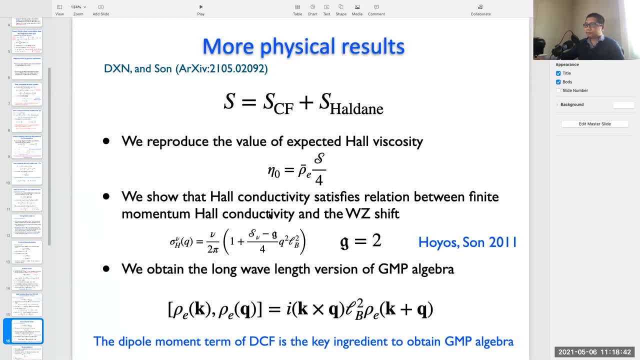 Wenzhen shift G-sheep. We also show that the Hohen connectivity satisfies the relation between the finite momentum Hohen connectivity and the Wen-G-sheep with this form, So basically for both nu. 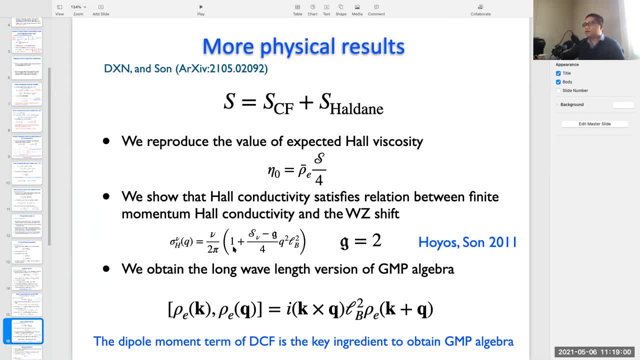 plus and nu minus, we have this equation satisfied, where S, nu is nothing but the Wen-G-sheep and G is the G-factor equal to 2.. And this relation was proposed by Kaloth-Huyos and Son in 2011.. So the result here suggests that our model satisfies the Galien invariant. 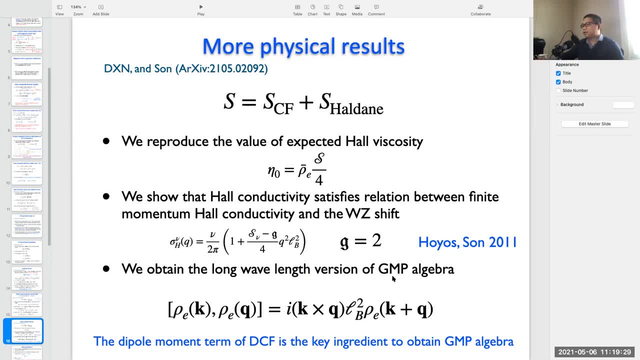 From this model we also obtain the long-wavelength version of GMP and Zebra, So the commutation duration of density with different momentum satisfies this equation. It's nothing but the long-wavelength limit of the GMP and Zebra, And we need to emphasize that. the dipole-moment terms that 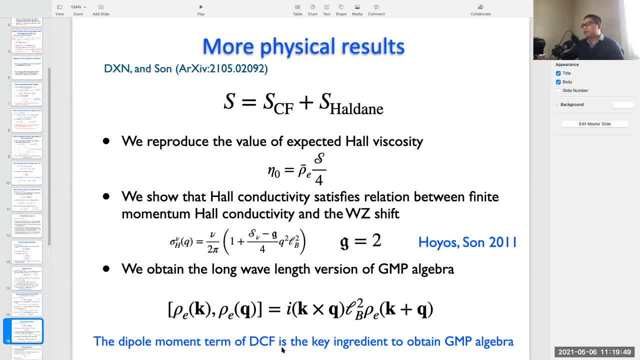 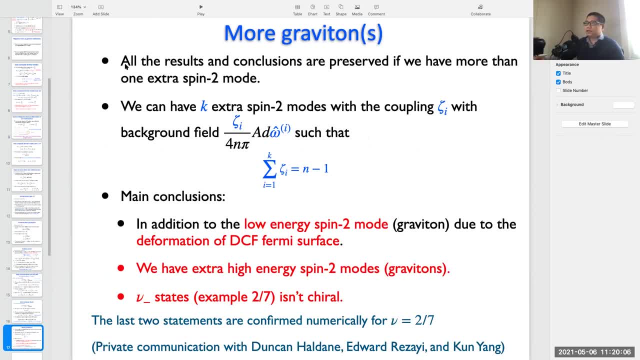 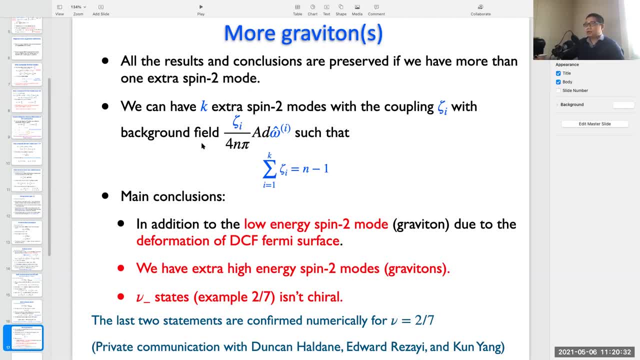 our model look so good. now us, on the previous result: satisfy: you have this condition for the coupling of the extra mode, And so one of the main conclusion of this talk is that we have the additional low energy. so, in addition to the low energy mode of spin 2 mode, which is the deformation, 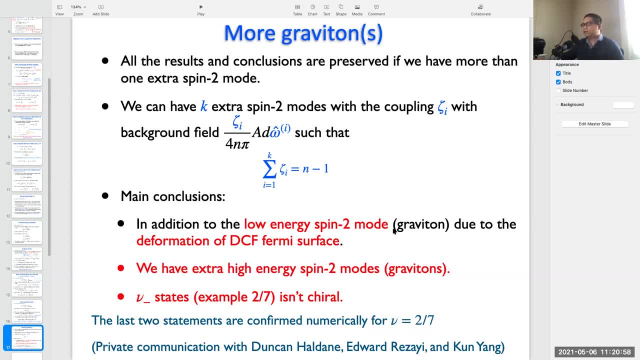 of the direct composite fermion surface we have extra spin 2 mode with higher energy And so we have more graviton mode. in the fractional quantum mode And also from the calculation of static structure factor we see that the new minor state doesn't saturate the Haldane bound. so that suggests that this: 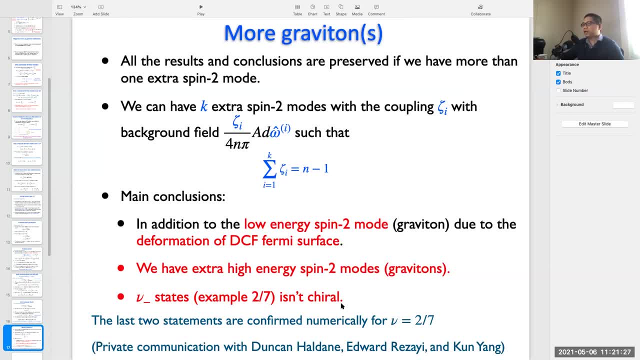 new minor state is in chiral, so we we will have more than one spin 2 mode and with a different chirality. And basically the last two statements are confirmed numerically for NU equal to 2.7 in the private communication with Duncan, Ed and Kunjang. 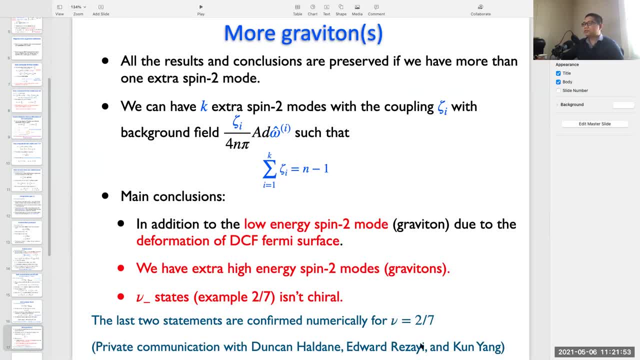 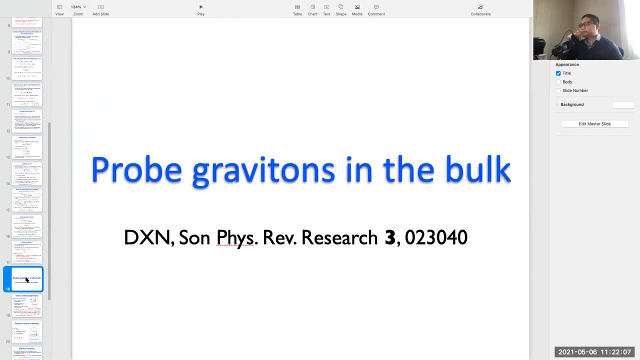 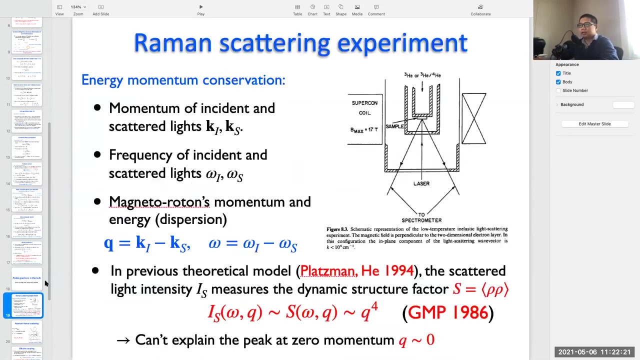 And let me take my chance to thank Ed to show us the numerical results that support our proposal and give us the confidence to publish the paper. So in the last part of my talk I will tell you how to probe the graviton using the Raman scattering experiment. So here is a set up of the Raman scattering. 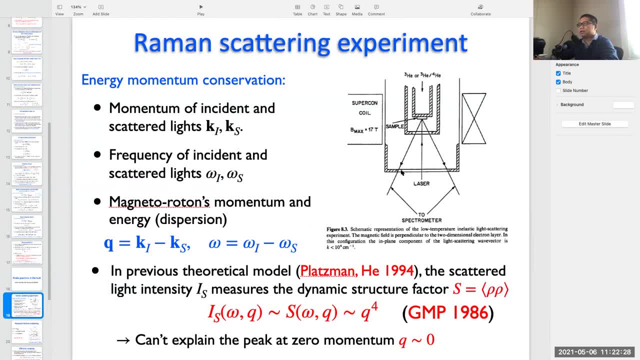 you have the sample here, the quantum hole sample. here You size the laser in and you measure the scatter photon, And from the momentum conservation and the energy conservation we can have the momentum of the excitation mode and also the frequency. So by measuring the scatter photon 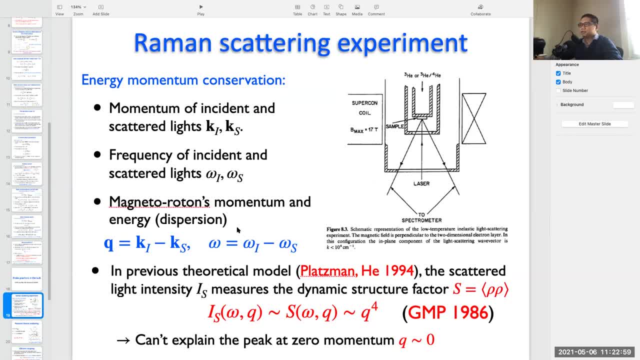 we can have the dispersion relation of the magnetroton mode And in the previous theoretical model by Flatman and he, the scatter light intensity is supposed to measure the dynamic structure factor. It's a density, density correlation function. However, you see that static structure factor. go to Q, to the fourth, 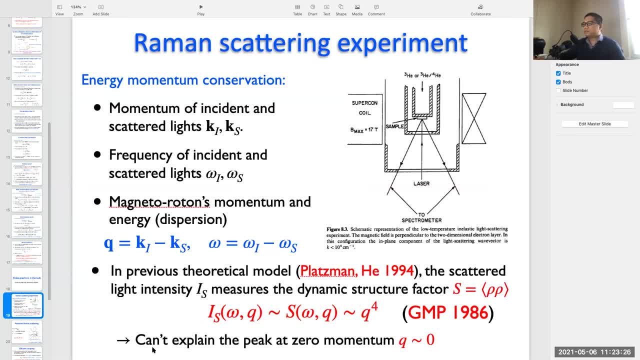 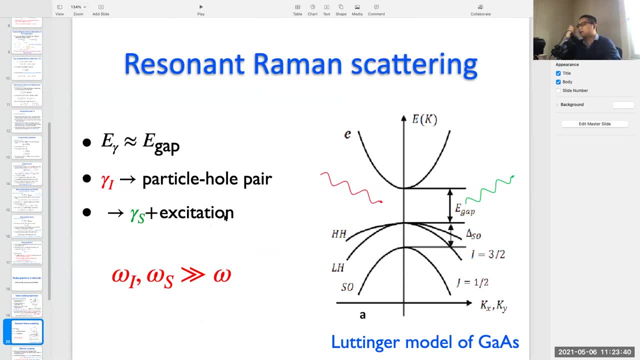 That means this theoretical model cannot explain the peak at zero momentum in the Raman scattering experiment. So together with CERN we propose a new model. So we study the model of photon coupled with both light hole and heavy holes, band and also electron band. 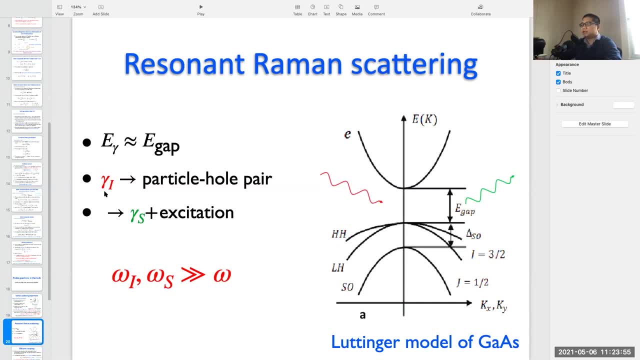 So we suggest that the photon come in. we excite the electron and hole pair. So electron here go up to the conducting band and give us the electron hole pair And after that the electron, the extra electron, will go down and emits the photon. So leave us proton excitation on the conducting band. 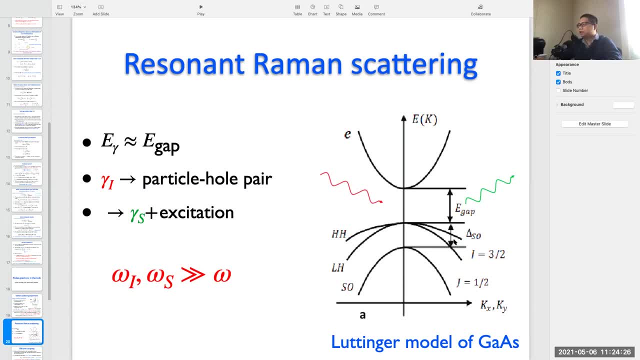 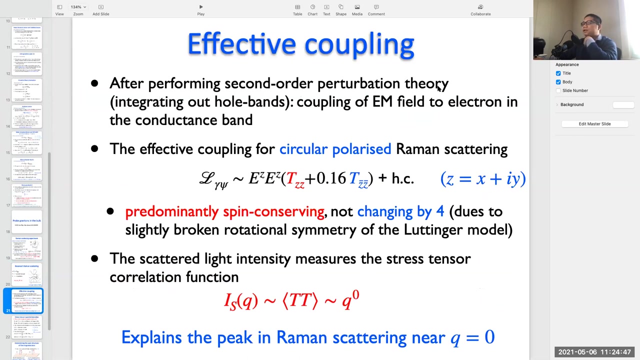 and give us back the full fill hole band And in the setup we consider the resonance scattering, where the frequency of photon should be very close to the energy gap between the conducting band and valent band, And after that we perform the second order perturbation theory by integrating our own of the whole band and we introduce 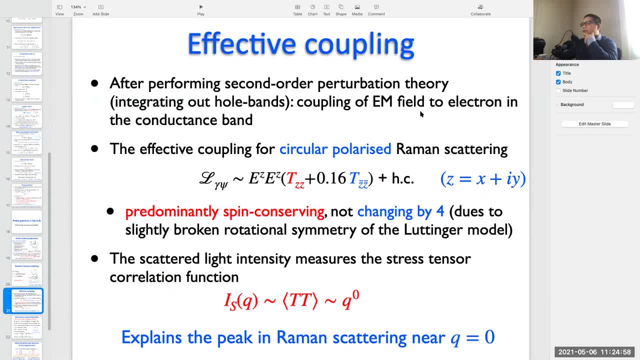 the epithetic coupling of the photon electromagnetic field to electron in the conductive band with this form, So TZZ and TZ bar. Z bar: here is nothing but it's a stress tensor in the in the conductive band and E is here is nothing but this electric field of photon. 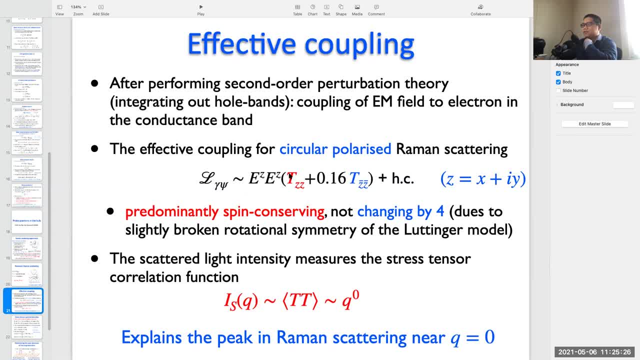 And here we have two terms, and the first term is rotational invariant and it's dominant. and the second term we have the, the term, the small term that violates the rotational invariant due to the broken rotational symmetry absoluting the model for the whole band. And in our effective model we we saw that the scatter light intensity measures, the 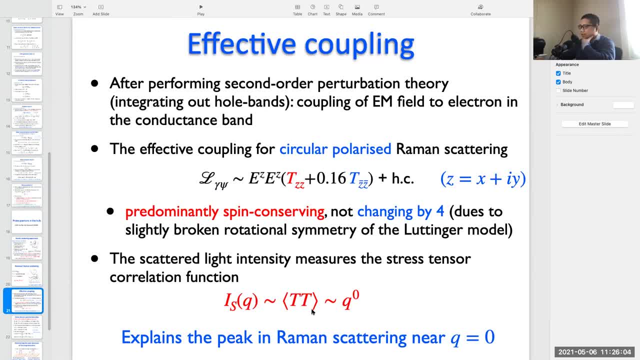 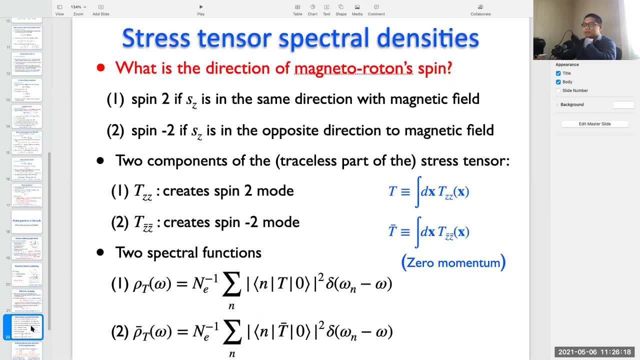 set tensor correlation function instead of the density density correlation function. So that means the model that we have proposed explains the peak in the Raman scattering near momentum equal to zero. So how much longer do you think you need? I think only if I have only three more slides and basically only. 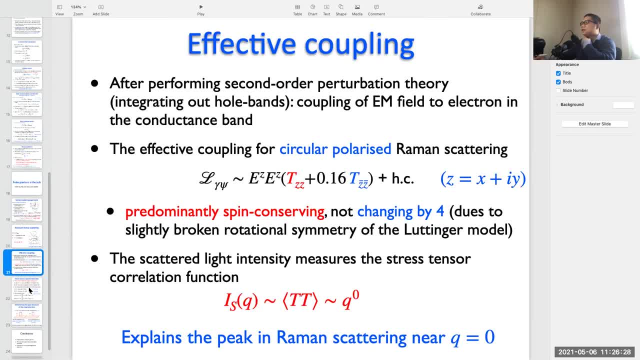 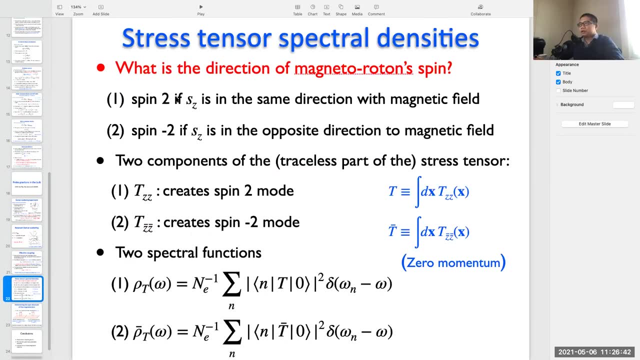 three, three, four minutes and I can finish. Okay, maybe if you could try to finish one or two minutes. Okay, I think it's fine, maybe because you can use some time over questions here. Yeah, yeah, sure, thank you. and basically we also propose that using Raman scattering, you not only can measure the dispersion duration, but 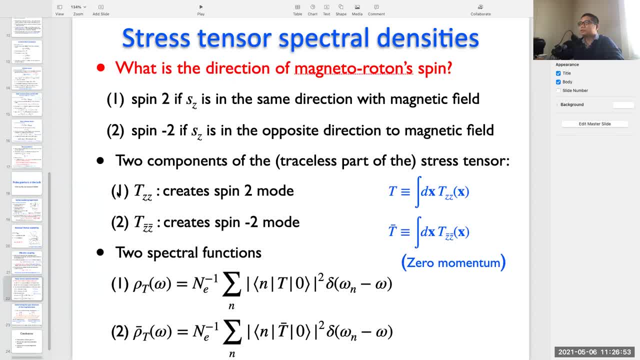 you also can measure the currentity of the spin two mode. So if we say that spin two excitation is spin two, if the z direction of the spin with the same direction with magnetic field, and you say that it's spin minus two if the spin in z direction is in the opposite direction to the magnetic field, 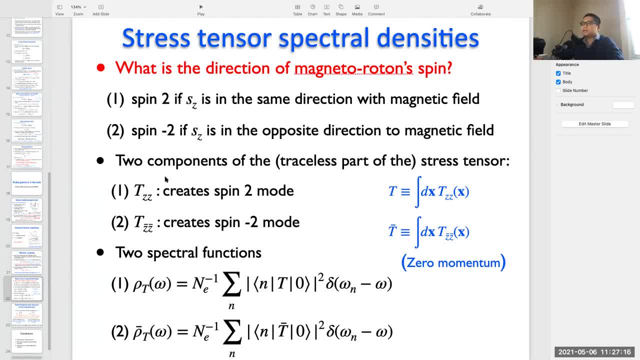 And basically we think that excitation would be induced by the action of the two components of the stress tensor, Tzz and Tzz bar. So that creates a spin two mode, and this one will increase the spin. And here we define the zero momentum of Tzz and Tz bar. 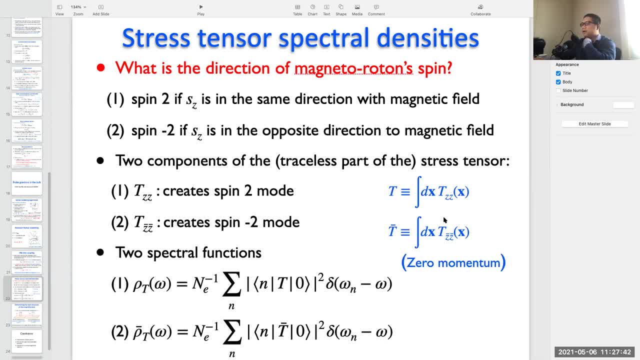 And so I mean this is given that if we add this forward and backward, so on the stream, if the production rate is T bar, And from that we have the definition of the two-spectral function. Yeah, it's a summation over the excitation. 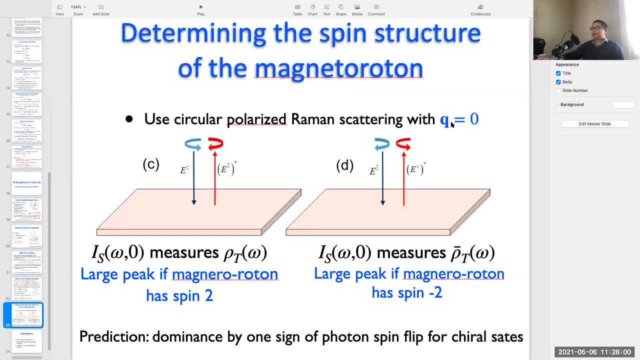 And with the circular polarity Raman scattering near q equal to zero, we saw that this experiment, the scatter line intensity, would measure the spectral function of Tzz And, with this opposite polarization, the scatter line intensity would measure the spectral function of the Tz bar, Z bar. 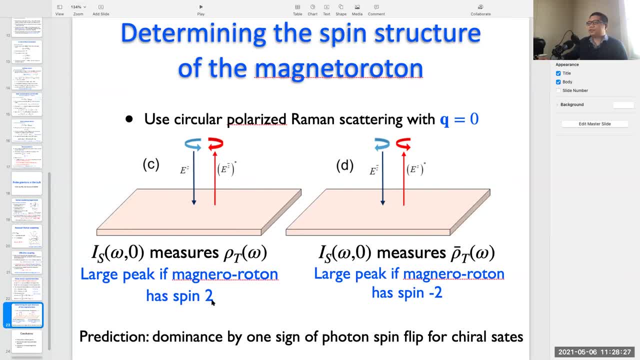 And we see that if the magnet of tone have the spin 2, then in this experiment we see a peak, the strong peak in this side. And if the magnet don't have the spin minus 2, then we see the strong peak on this side. So for the current state, we see that the result will dominate by one side of photon. 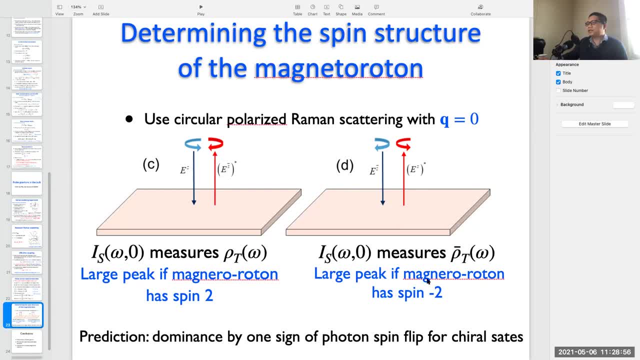 spin flip. So either this side or this side we see the strong peak And from that we can show that. if measure the spectral function here we see that if we have more than one peak at a different frequency and we can say that we have more than one, 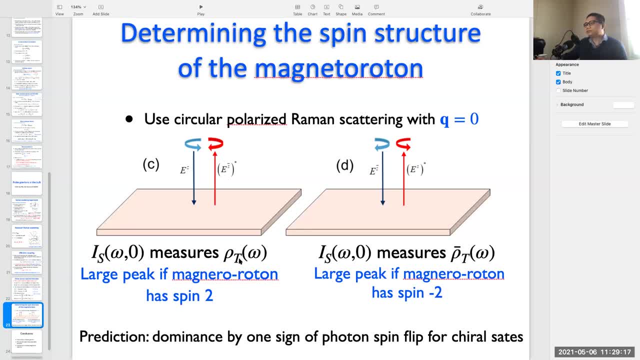 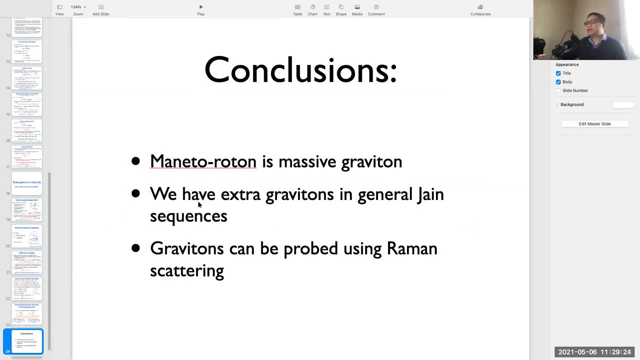 force more than one graviton. And let me go to my conclusion. So in this talk I show that magnetotone is a massive graviton and we have extra gravitons in general gain sequence near 1 fractилs per unit time-raum. 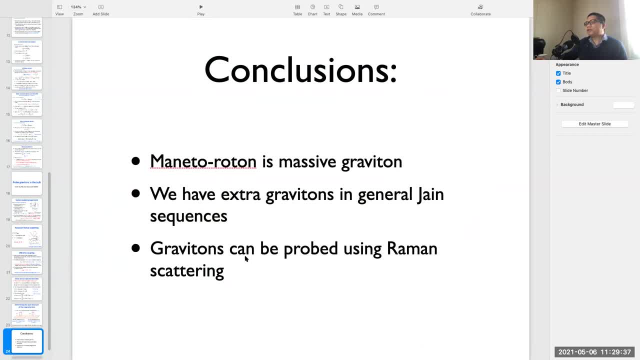 in tetra and the graviton can be probed using the circular pori-Riemann scattering. Thank you, Thank you, clap. on behalf of the audience. Yeah, so now questions for both Sung and Lauren. please raise your hand.